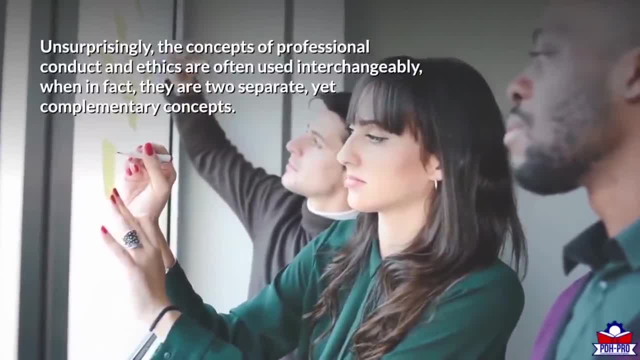 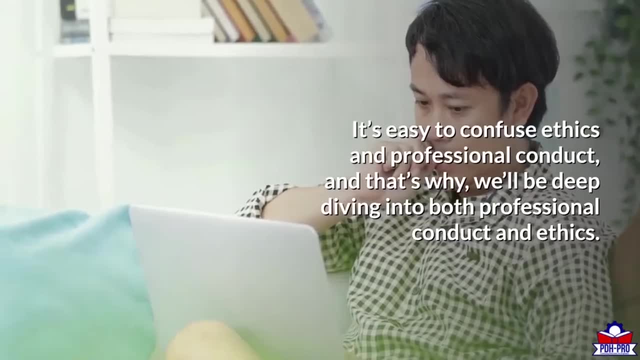 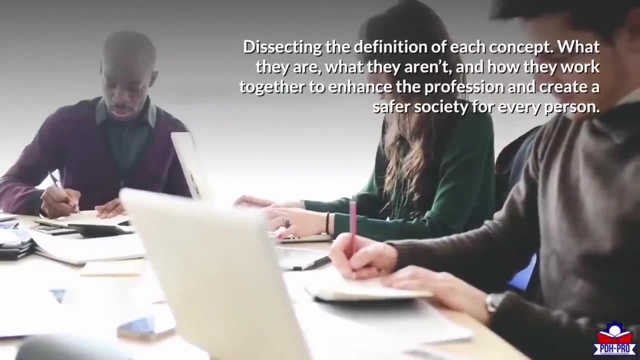 are often used interchangeably when in fact they are two separate yet complementary concepts. It's easy to confuse ethics and professional conduct, and that's why we'll be deep diving into both professional conduct and ethics, Dissecting the definition of each concept, what they are, what they aren't and how they. 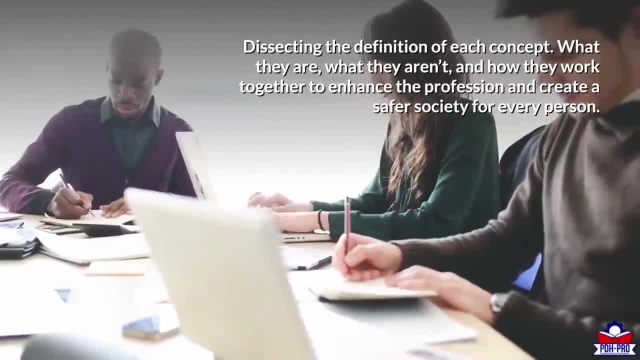 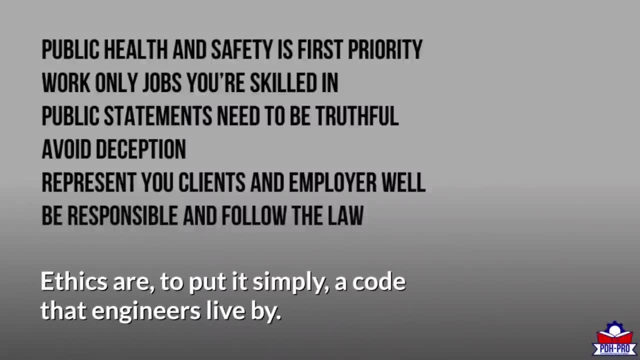 work together to enhance the profession and create a safer society for every person. What do we mean by ethics? Ethics are, to put it simply, a code that engineers live by. A code of ethics functions like a statement of values for a company or organization In 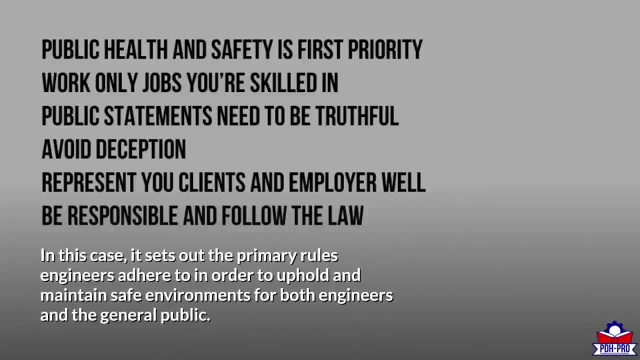 this case, it sets out the primary rules engineers adhere to in order to uphold and maintain safe environments for both engineers and professionals. This code of ethics is used by engineers and the general public Because the trust and confidence the public has in engineering rests upon complete adherence to ethical behavior. keeping this code is a major priority. 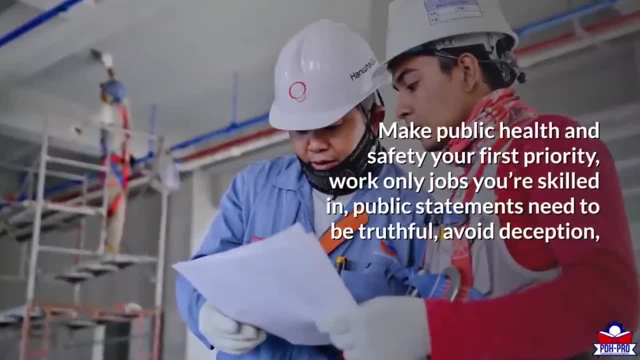 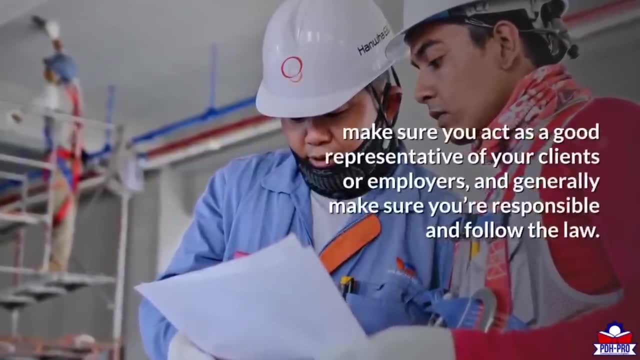 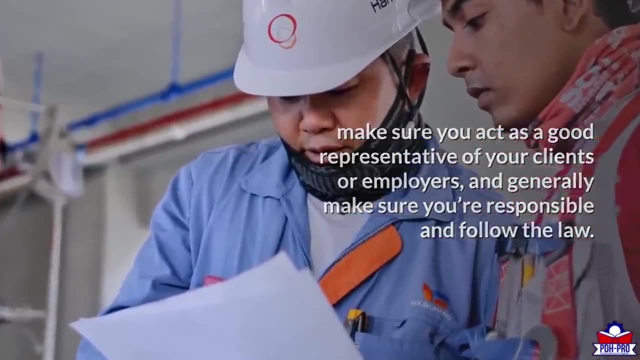 You know the general code of ethics. Make public health and safety your first priority. Work only jobs you're skilled in. Public statements need to be truthful. Avoid deception. Make sure you act as a good representative of your clients or employers and generally make sure you're responsible and follow the law. 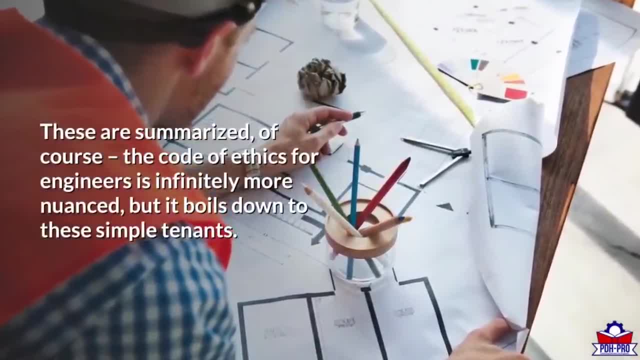 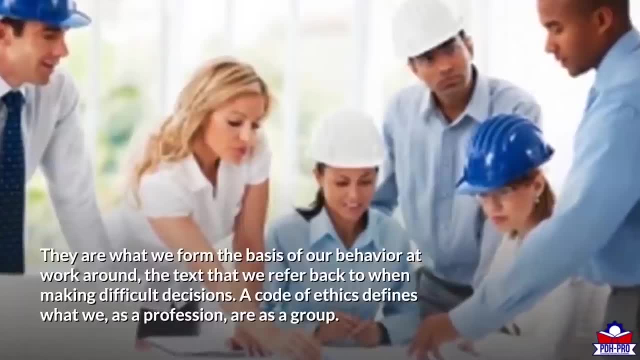 Summarized. of course, the code of ethics for engineers is infinitely more nuanced, But it boils down to these simple tenets. They are what we form, the basis of our behavior at work around, the text that we refer back to when making difficult decisions: A code, 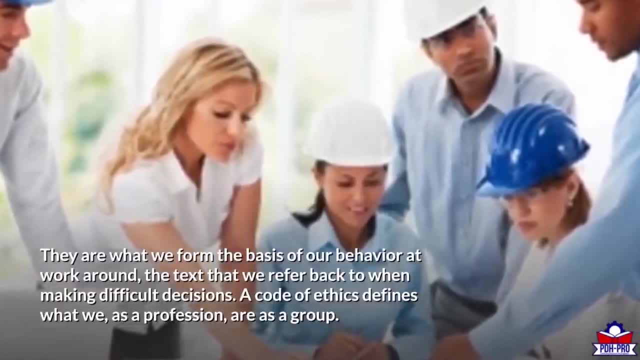 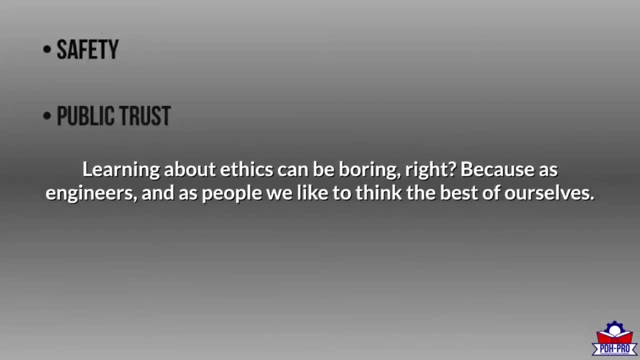 of ethics defines what we as a profession are as a group. Why are ethics important? Learning about ethics can be boring, right, Because, as engineers and as people, we like to think the best of ourselves. We all love to believe that we're. 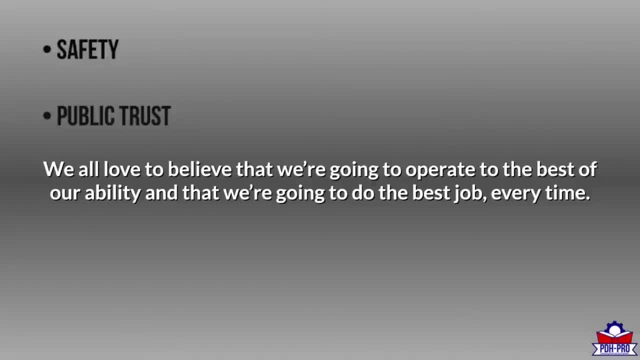 going to operate to the best of our ability and that we're going to do the best job. every time, The code of ethics seems like the terms of service on a website, something we scroll past in order to get to the good stuff. Unfortunately, situations can arise. 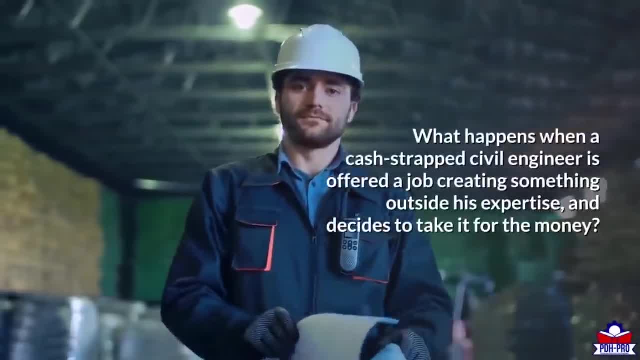 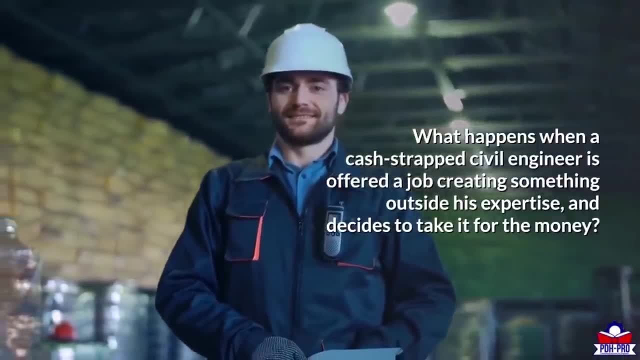 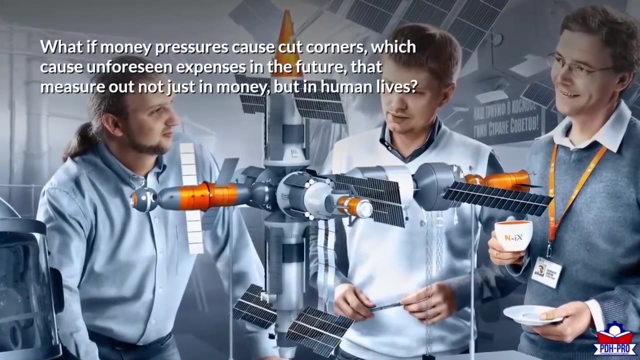 that put us in difficult situations. What happens when a cash-strapped, simple engineer is offered a job creating something outside his expertise and decides to take it for the money? Will the end product be of good quality or even safe? What if money pressures cause cut corners which cause unforeseen expenses in the future? 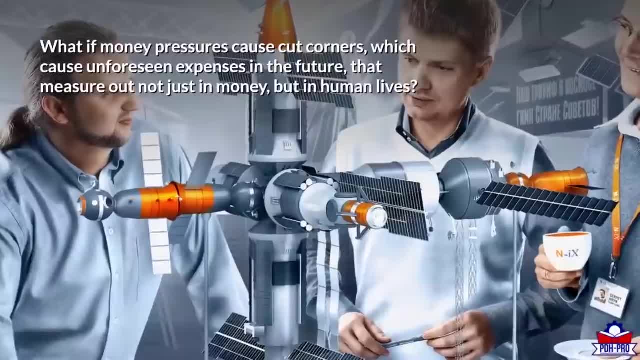 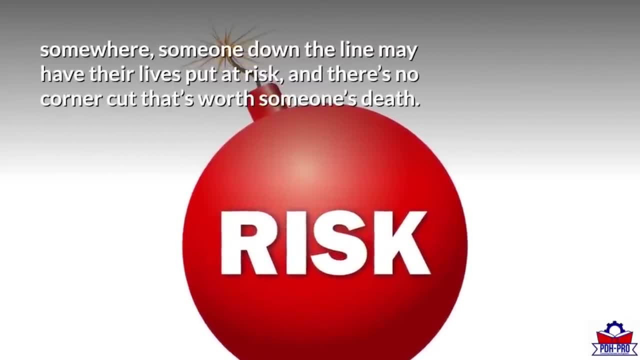 that measure out not just in money but in human lives. To put it simply and brutally: if we don't do our job by the code of ethics set down somewhere, someone down the line may have their lives put at risk, and there's no corner. 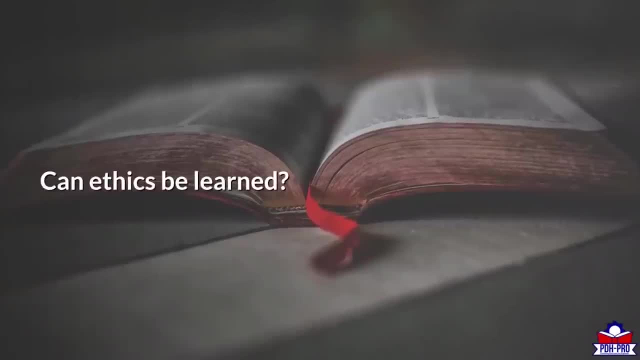 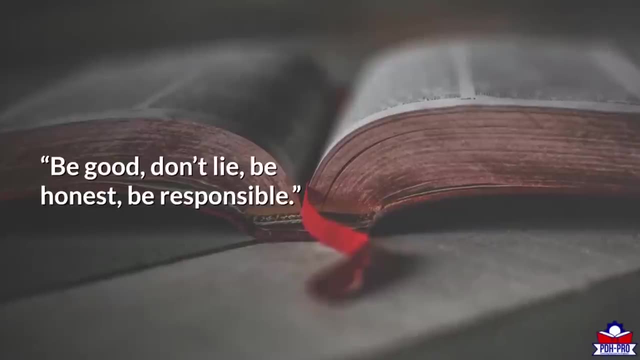 cut. that's worth someone's death. Can ethics be learned? At first glance, a code of ethics reads like a list of personality traits. doesn't it Be good? Don't lie, Be honest. Don't be honest, Be responsible. These traits do come easier to some than to others, and it has. 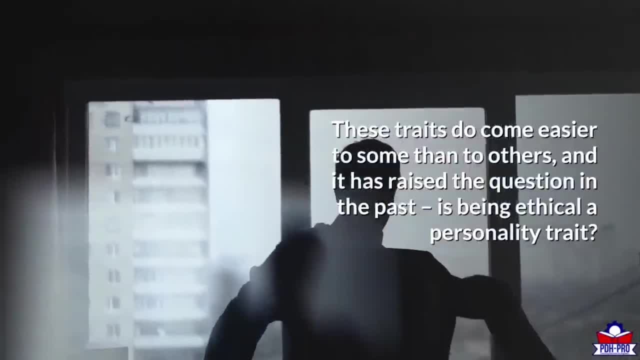 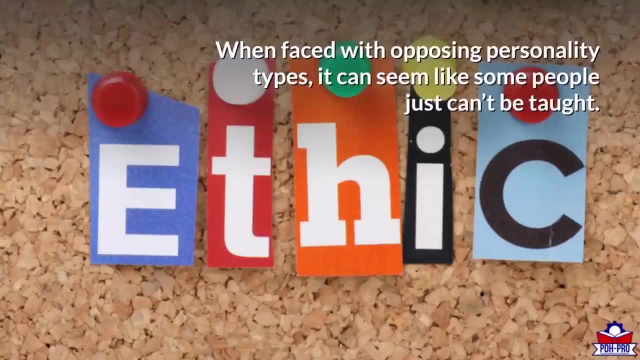 raised the question in the past: is being ethical a personality trait? Can a person really be taught to adhere to ethical principles When faced with opposing personality types? it can seem like some people just can't be taught After all. it seems that deep down. 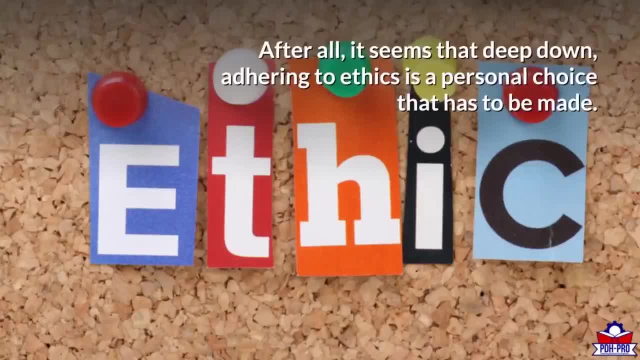 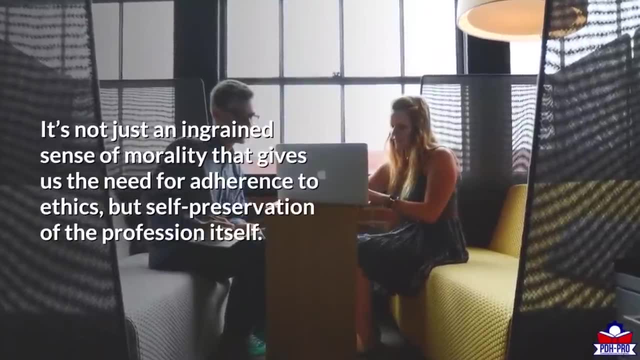 adhering to ethics is a personal choice that has to be made. There are arguments, though, that could be made on the teaching of ethical behavior. It's not just an ingrained sense of morality that gives us the need for adherence to ethics. 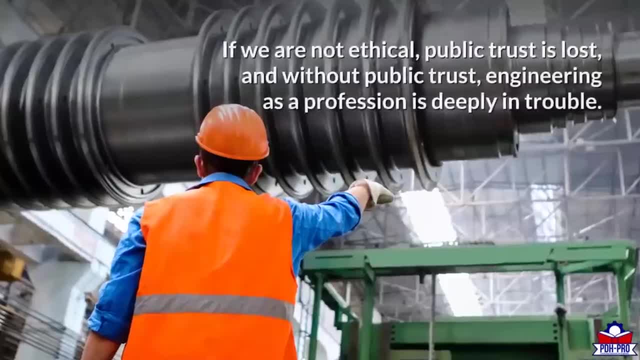 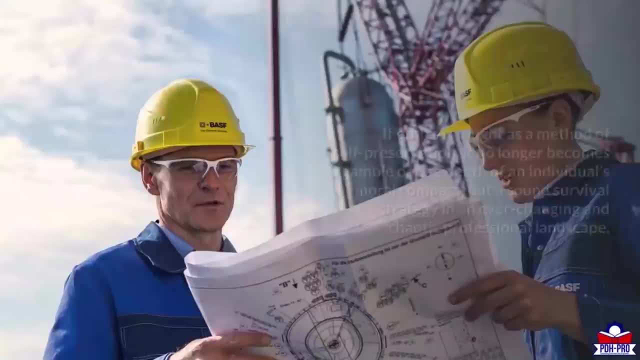 but self-preservation of the profession itself. If we are not ethical, public trust is lost, and without public trust, engineering as a profession is deeply in trouble. If ethics is taught as a method of self-preservation, it no longer becomes a gamble on the depth. 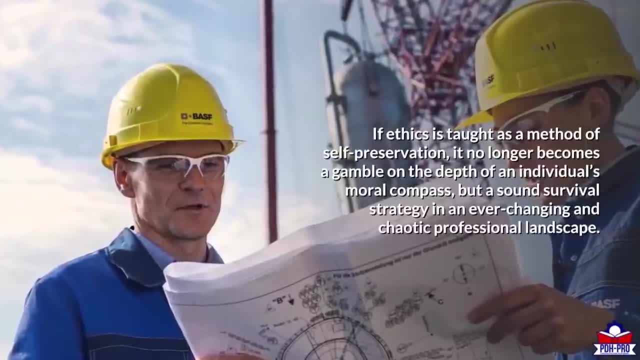 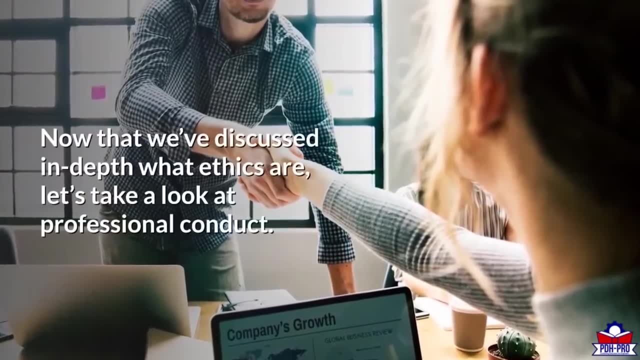 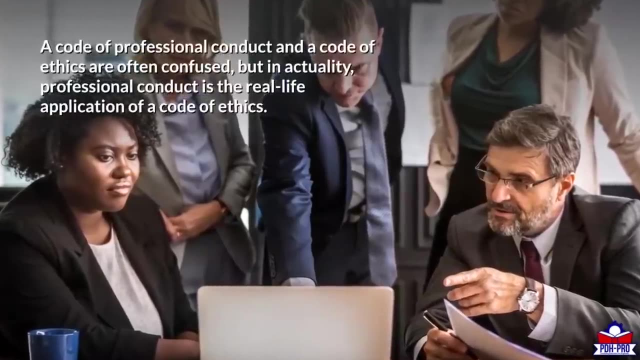 of an individual's moral compass, but a sound survival strategy in an ever-changing and chaotic professional landscape. What is professional conduct? Now that we've discussed in-depth what ethics are, let's take a look at professional conduct. A code of professional conduct and a code of ethics are often confused, but in actuality, 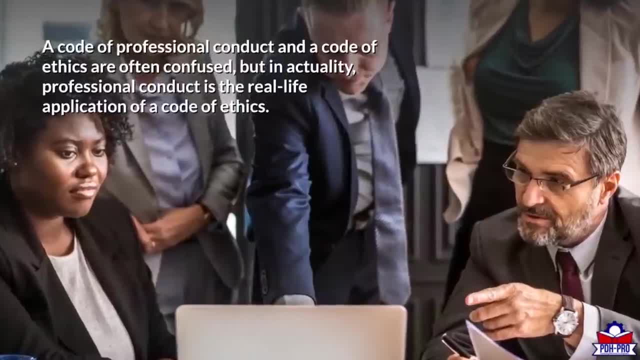 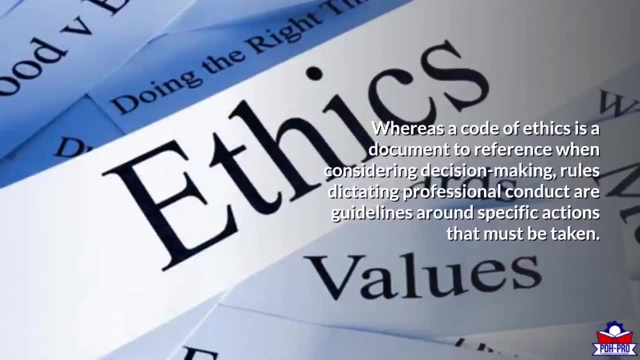 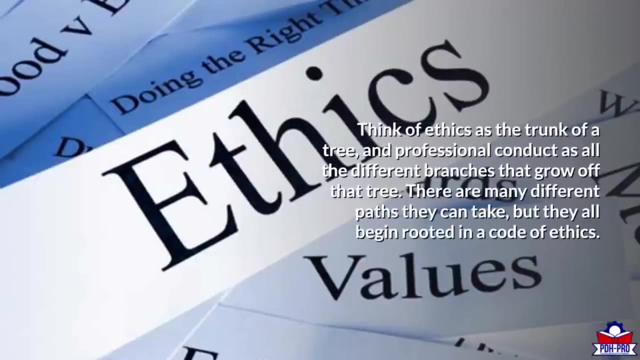 professional conduct is the real-life application of a code of ethics, Whereas a code of ethics is a document to reference when considering decision-making. rules dictating professional conduct are guidelines around specific actions that must be taken. Think of ethics as the trunk of a tree and professional conduct as all the 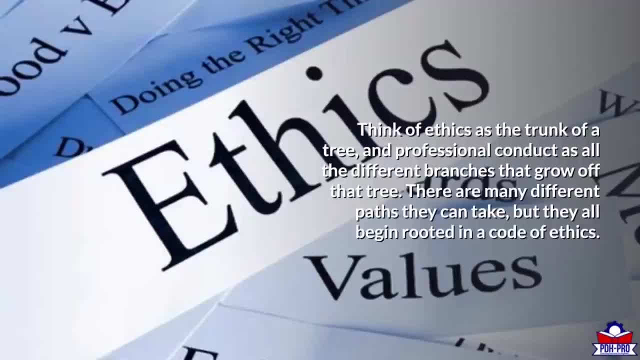 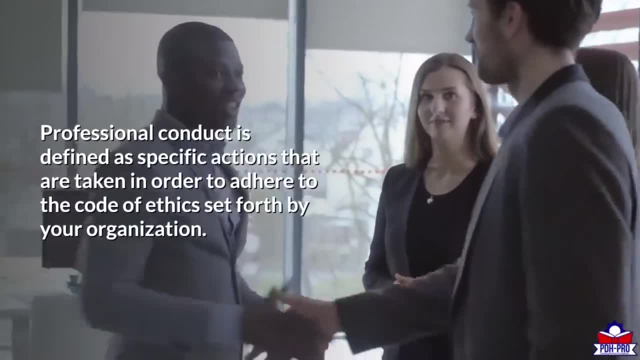 different branches that grow off that tree. There are many different paths they can take, but they all begin rooted in a code of ethics. Professional conduct is defined as specific actions that are taken in order to adhere to the code of ethics set forth by your organization. 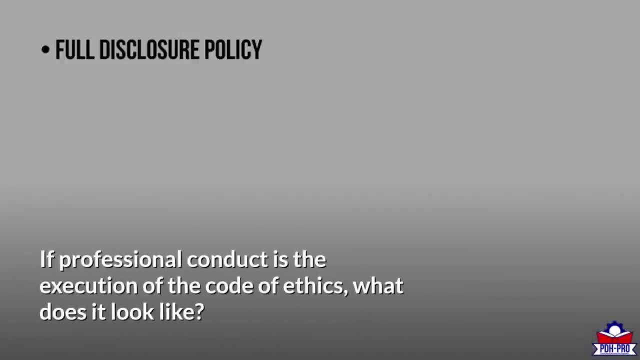 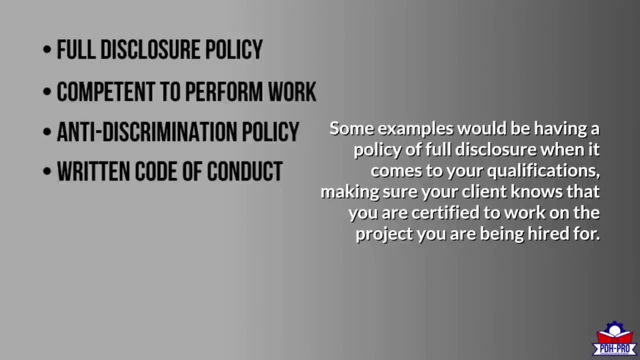 What are some examples of professional conduct? If professional conduct is the execution of the code of ethics, what does it look like? Some examples would be: having a policy of full disclosure when it comes to your qualifications, making sure your client knows that you are certified to work on the project you are. 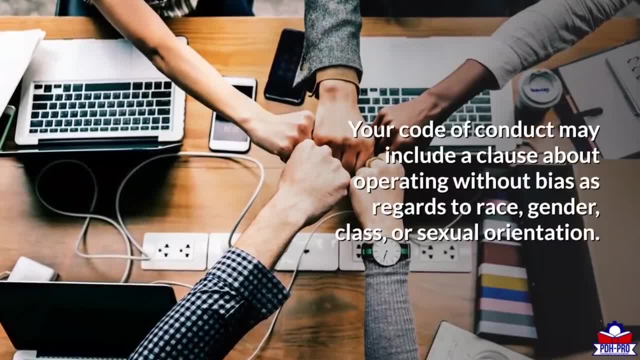 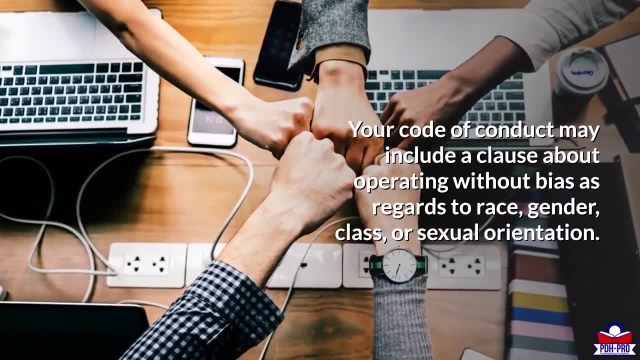 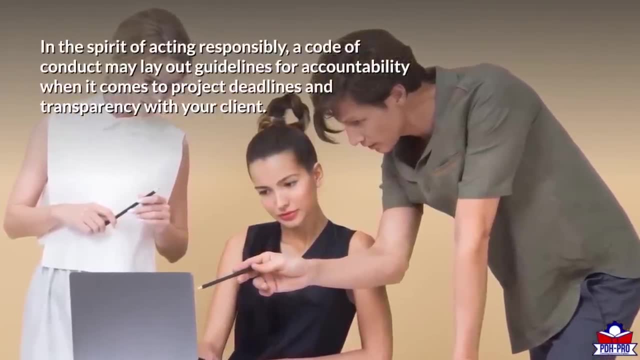 being hired for. Your code of conduct may include a clause about operating without bias as regards to race, gender, class or sexual orientation. In the spirit of acting responsibly, a code of conduct may lay out guidelines for accountability when it comes to project deadlines and transparency with your client. 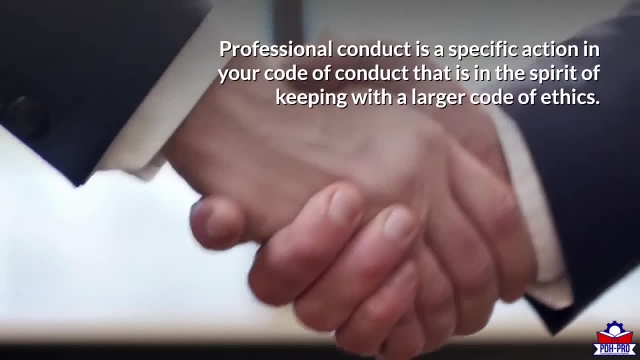 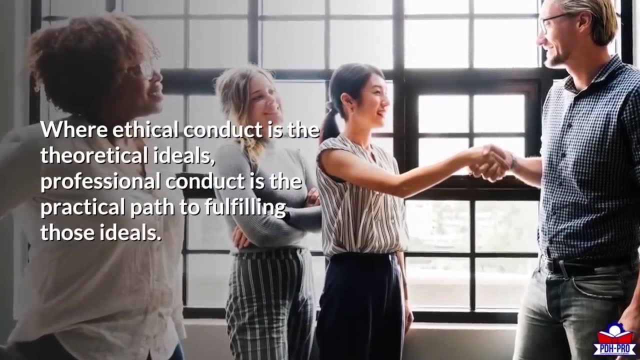 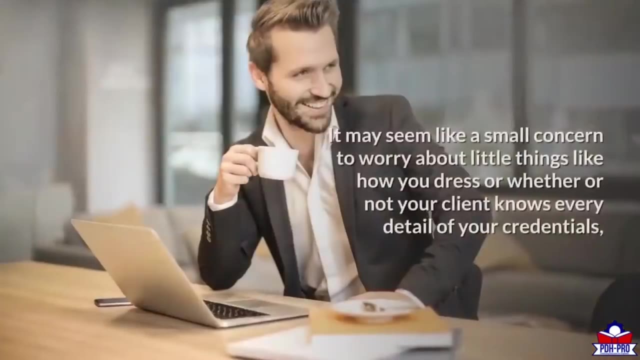 Professional conduct is a specific action in your code of conduct that is in the spirit of keeping with a larger code of conduct Where ethical conduct is the theoretical ideals. professional conduct is the practical path to fulfilling those ideals. How does behavior influence perception? It may seem like a small concern to worry about little things like how you dress or 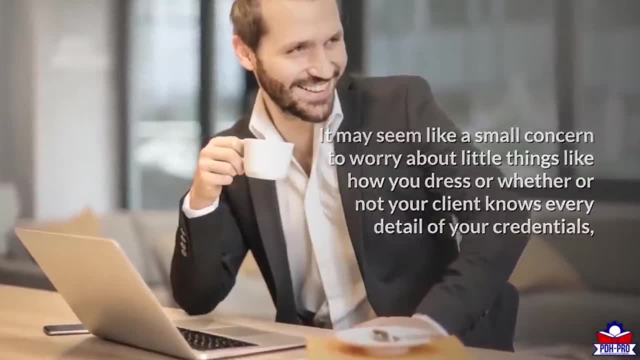 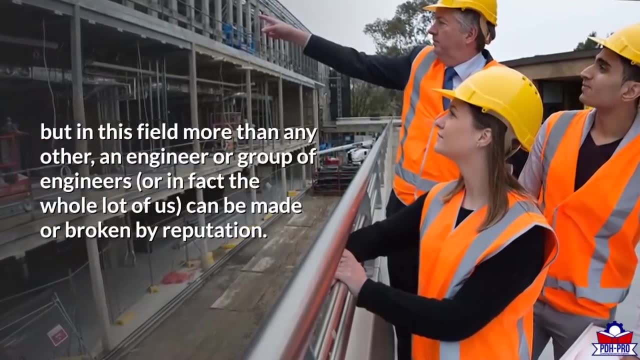 whether or not your client knows every detail of your credentials. But in this field, more than any other, an engineer or group of engineers, or in fact, the whole lot of us, can be made or broken by reputation. The more you see your reputation as an asset, the more likely you are to be a failure. 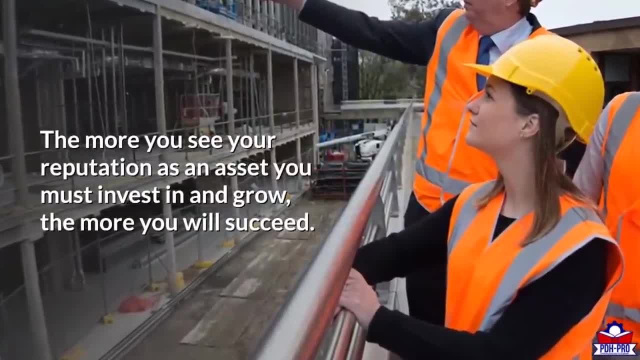 The more you see your reputation as an asset, the more likely you are to be a failure, And the higher an asset you must invest in and grow, the more you will succeed. You may think a dress code is a small thing, but dressing and acting professionally can. 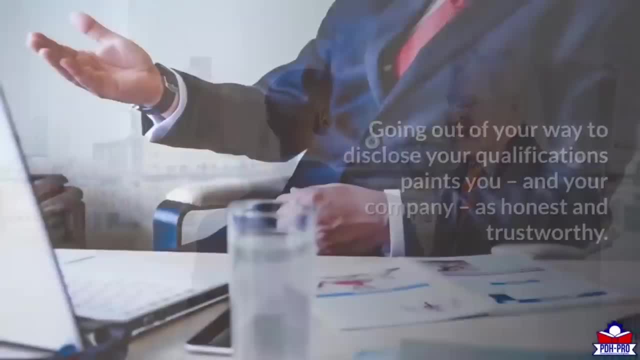 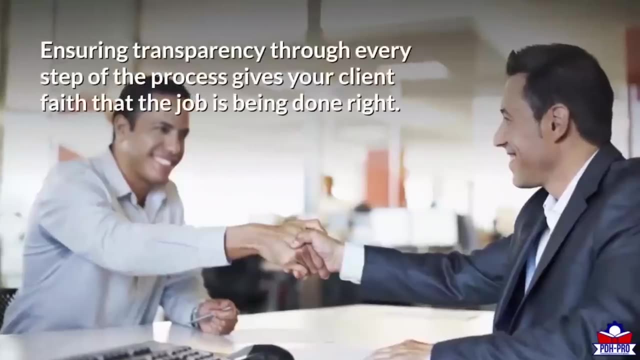 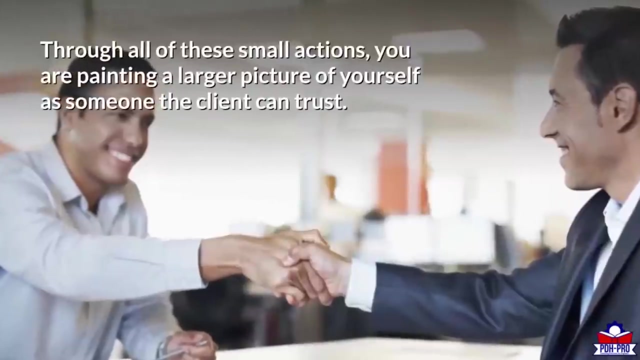 grow your impression as responsible and reliable. Going out of your way to disclose your qualifications paints you and your company as honest and trustworthy. Ensuring transparency through every step of the process gives your client faith that the job is being done. right Through all of these small actions, you are painting a larger picture of yourself as someone. 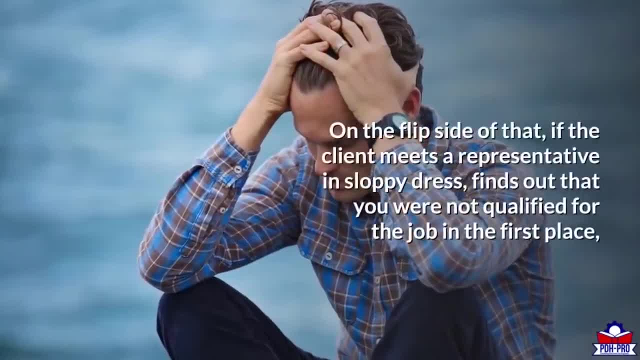 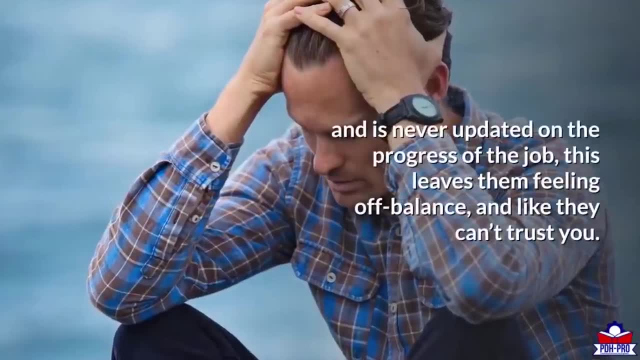 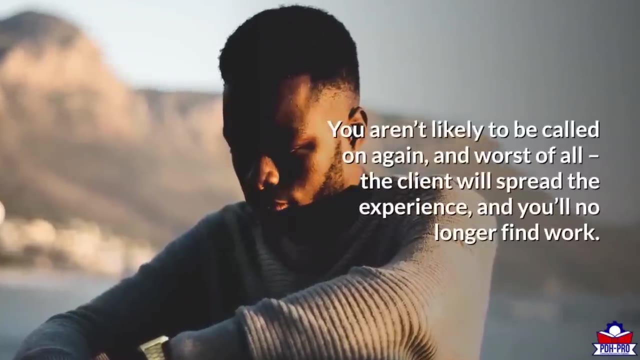 can trust. On the flip side of that, if the client meets a representative in sloppy dress, finds out that you were not qualified for the job in the first place and is never updated on the progress of the job, this leaves them feeling off balance and like they can't trust you. You aren't likely to be called on again. 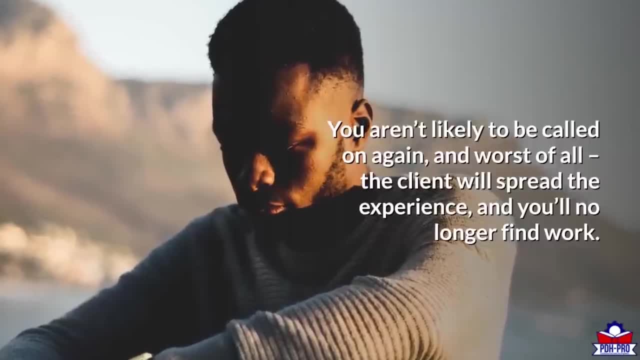 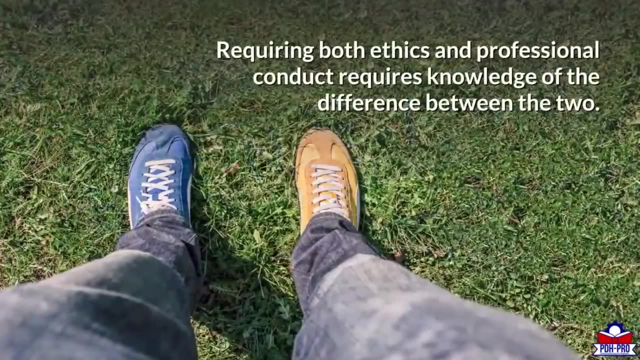 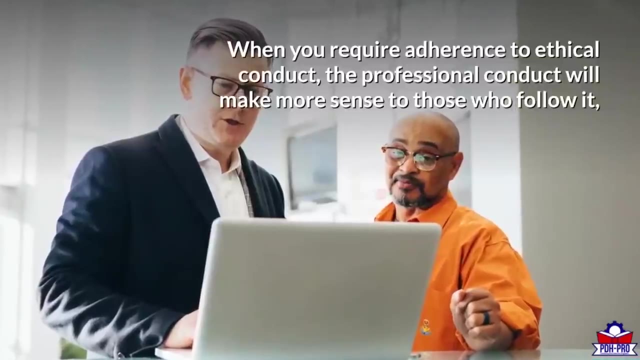 and, worst of all, the client will spread the experience and you'll no longer find work. What is the benefit of requiring professional conduct and ethics? Requiring both ethics and professional conduct requires knowledge of the difference between the two. When you require adherence to ethical conduct, the 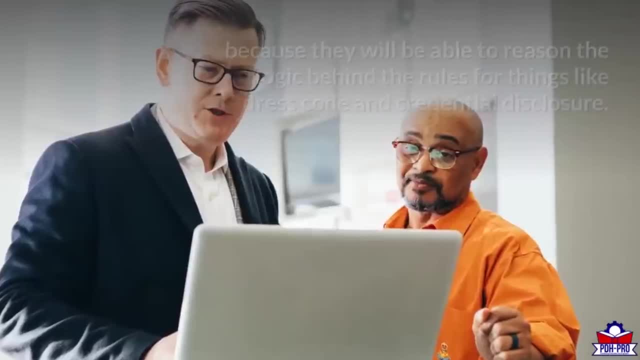 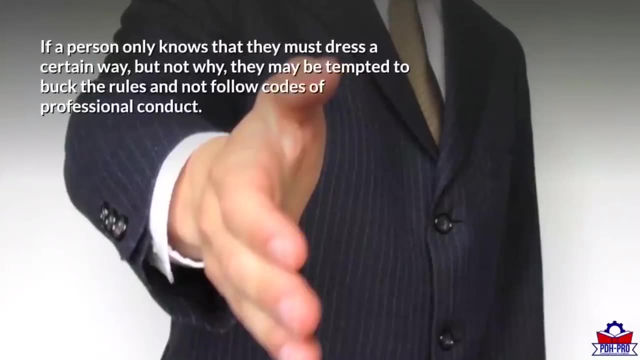 professional conduct will make more sense to those who follow it, because they will be able to reason the logic behind the rules for things like dress code and credential disclosure. If a person only knows they must dress a certain way, but not why, they may be tempted to buck the rules and not follow. 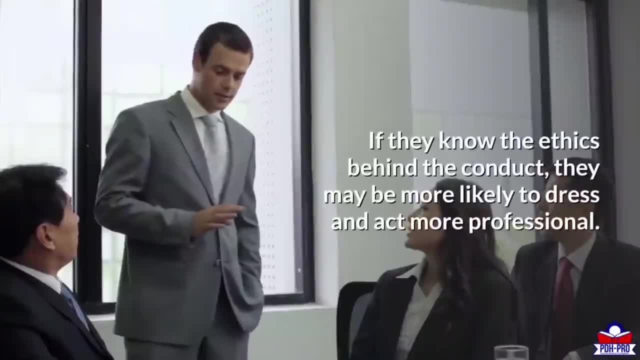 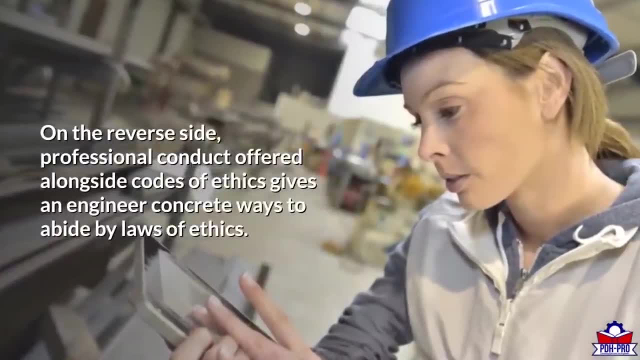 codes of professional conduct. If they know the ethics behind the conduct conduct, they may be more likely to dress and act more professional. On the reverse side, professional conduct offered alongside codes of ethics gives an engineer concrete ways to abide by laws of ethics. 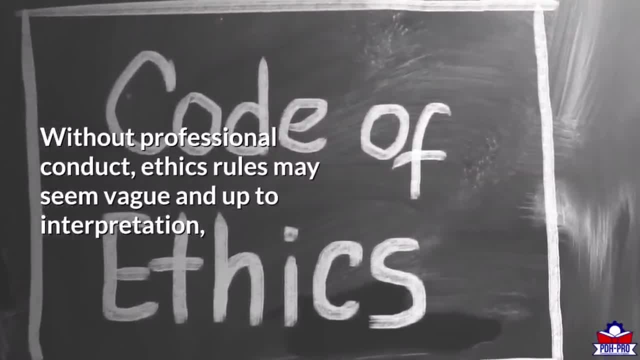 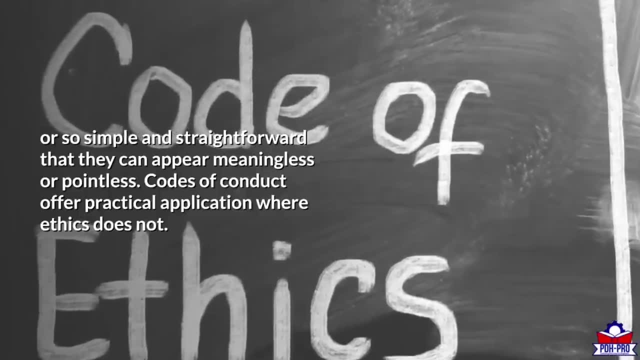 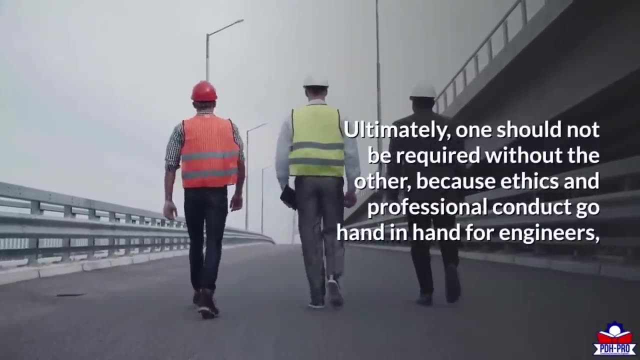 Without professional conduct, ethics rules may seem vague and up to interpretation, or so simple and straightforward that they can appear meaningless or pointless. Codes of conduct offer practical application where ethics does not. Ultimately, one should not be required without the other, because ethics and professional 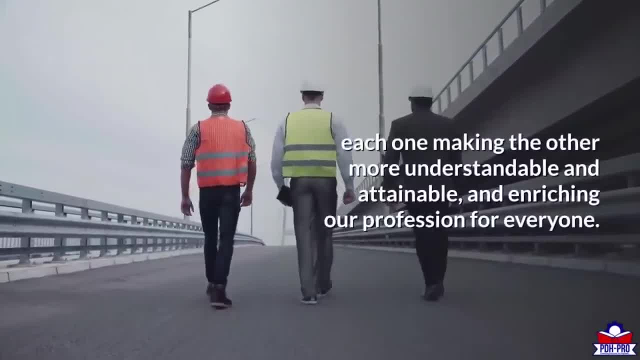 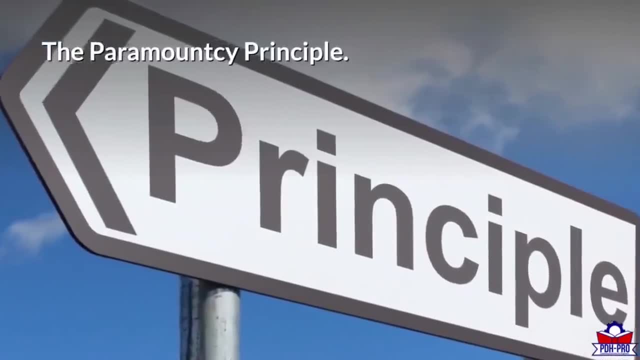 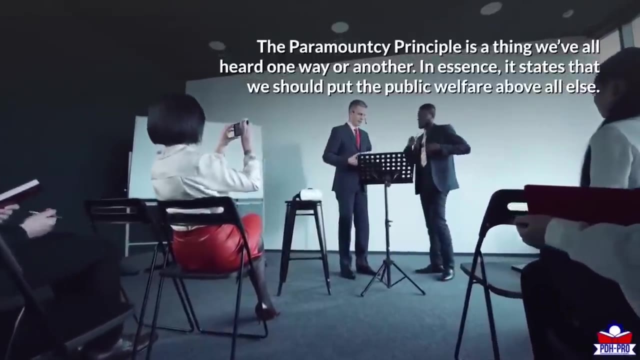 conduct go hand in hand for engineers, each one making the other more understandable and attainable and enriching our profession for everyone. The Paramountcy Principle. The Paramountcy Principle is a thing that we've all heard one way or another. In essence, it states that we should put the public welfare above all else. 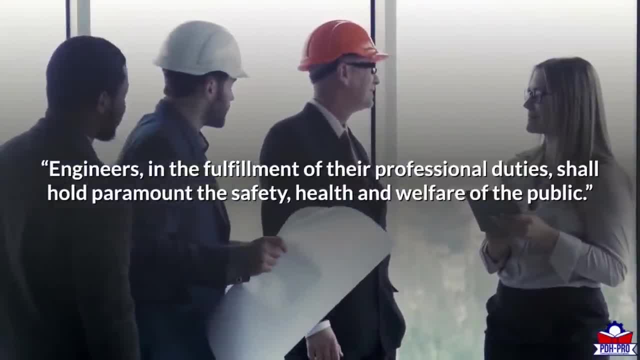 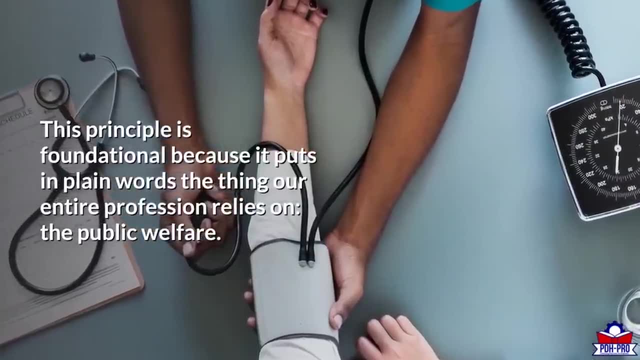 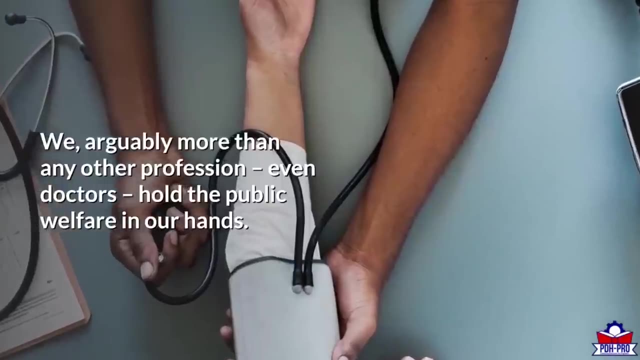 Engineers, in the fulfillment of their professional duties, shall hold paramount the safety, health and welfare of their employees. This principle is foundational because it puts in plain words the thing our entire profession relies on: the public welfare. We arguably more than any other profession- even doctors- hold the public welfare in our 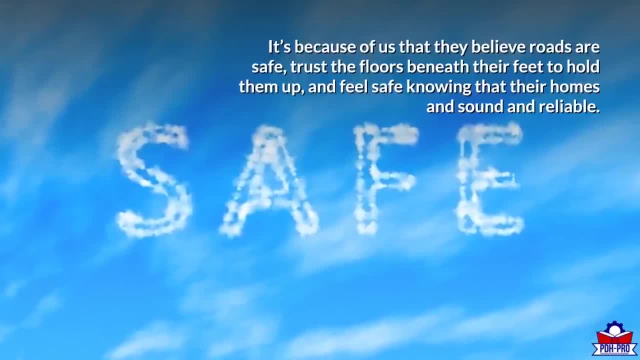 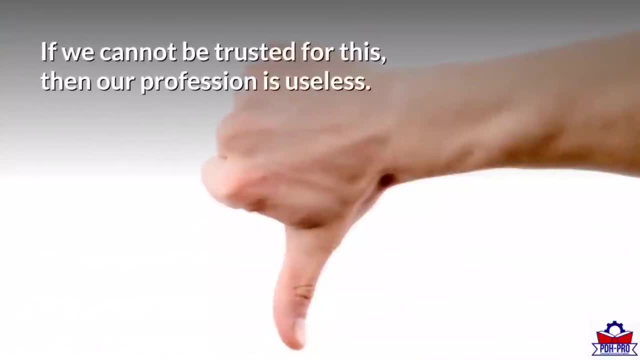 hands. It's because of us they believe roads are safe, trust the floors beneath their feet to hold them up and feel safe knowing that their homes are sound and reliable. If we cannot be trusted for this, then our profession is useless. In many ways, the Paramount Principle is the same. 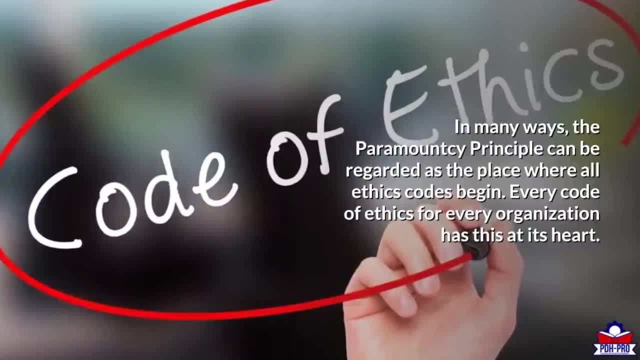 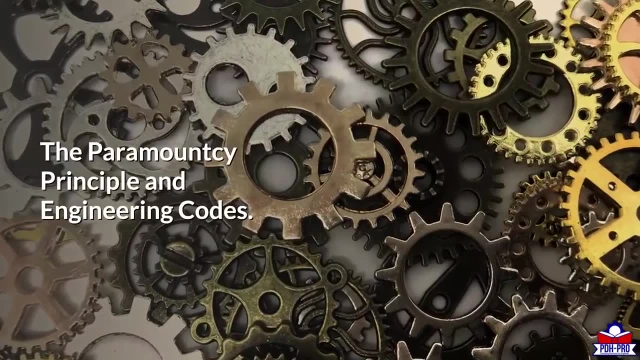 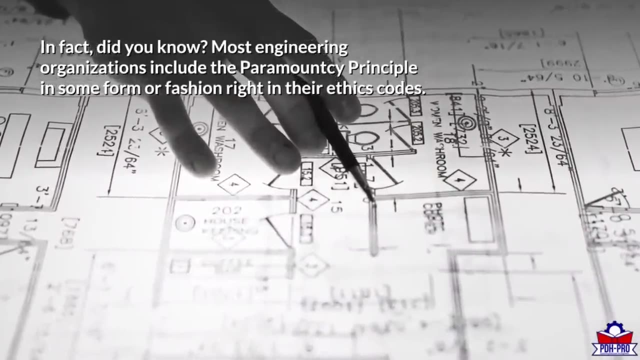 The Paramount Principle can be regarded as the place where all ethics codes begin. Every code of ethics for every organization has this at its heart: The Paramountcy Principle and Engineering Codes. In fact, did you know? most engineering organizations include the Paramountcy Principle in some. 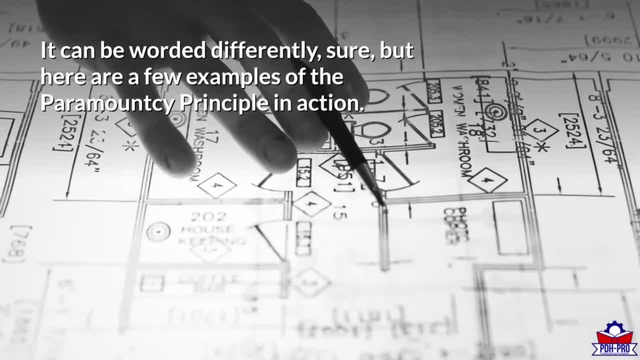 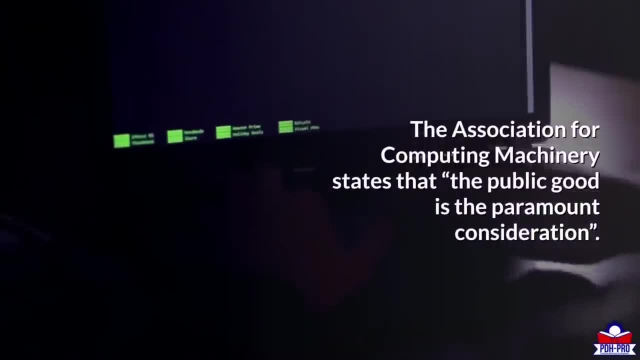 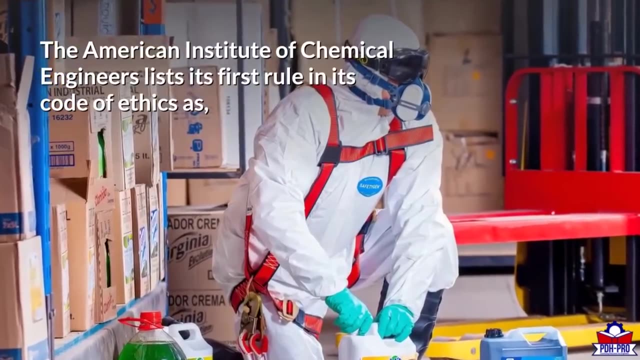 form or fashion right in their ethics codes. It can be worded differently, sure, But here are a few examples of the Paramountcy Principle. in action, machinery states that the public good is the paramount consideration. the american institute of chemical engineers lists its first rule in its code of ethics as hold paramount: the safety, health. 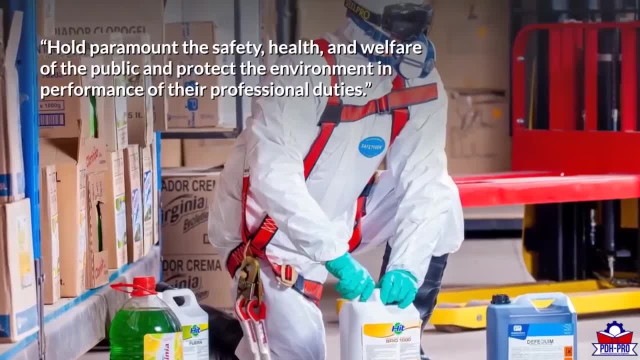 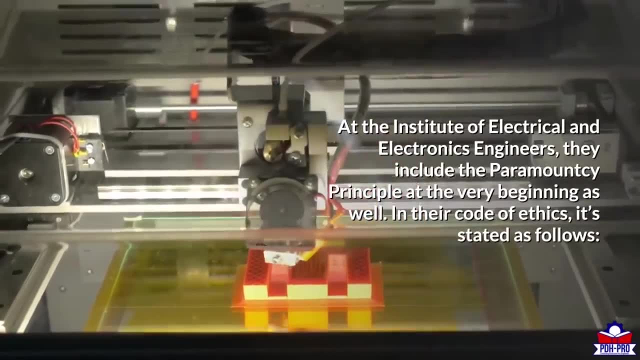 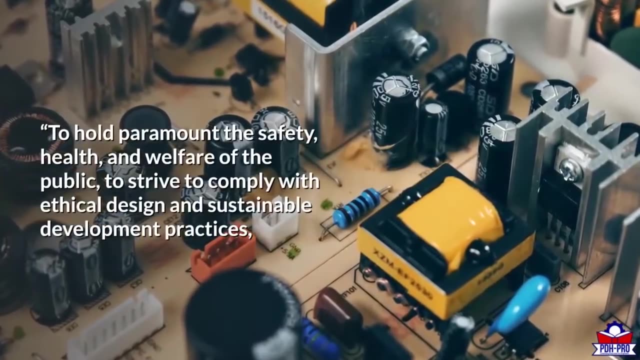 and welfare of the public and protect the environment. in performance of their professional duties at the institute of electrical and electronics engineers, they include the paramount principle at the very beginning as well. in their code of ethics it stated as follows: to hold paramount the safety, health and welfare of the public. to strive to comply with ethical design. 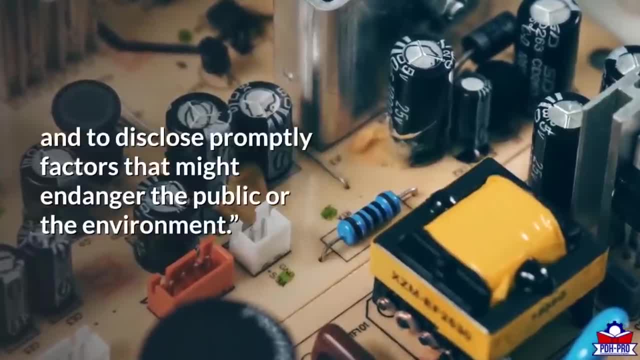 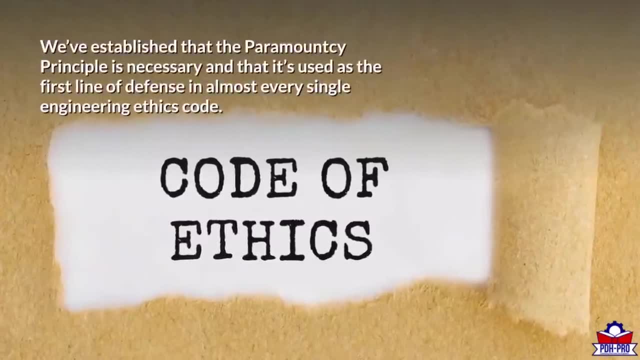 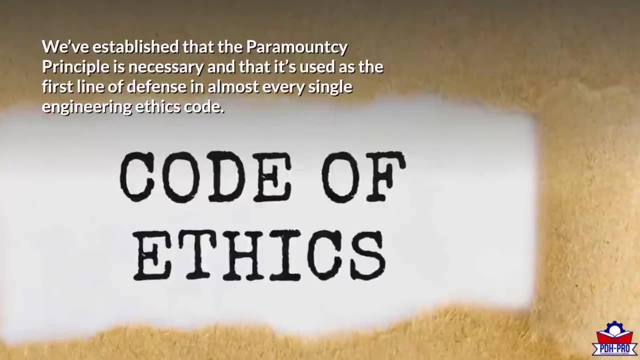 and sustainable development practices and to disclose promptly factors that might endanger the public or the environment. how is this principle relevant? we've established that the paramount c principle is necessary and that it's used as the first line of defense in almost every single engineering ethics code. but let's break down what it means for ethics. 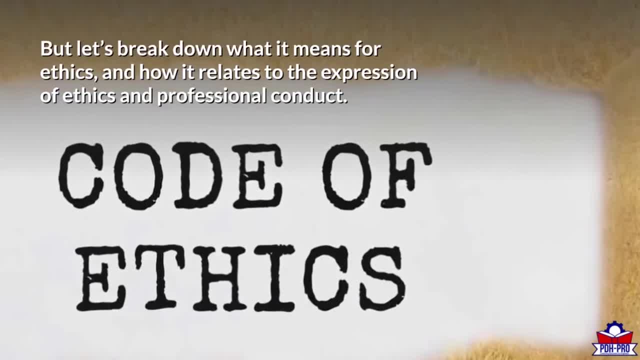 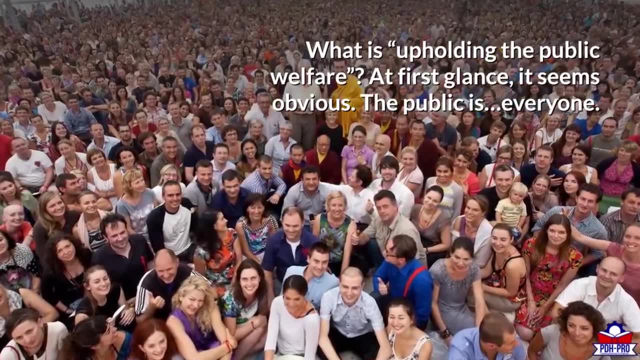 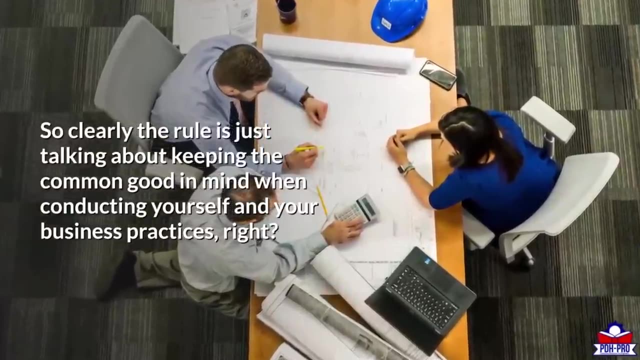 and how it relates to the expression of ethics and professional conduct. what is upholding the public welfare? at first glance, it seems obvious. the public is everyone, so clearly the rule is just talking about keeping the common good in mind when conducting yourself and your business practices. right, well, yes, but there may be a few hidden implications that not 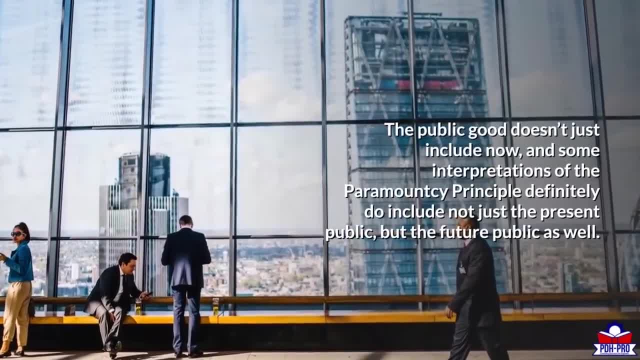 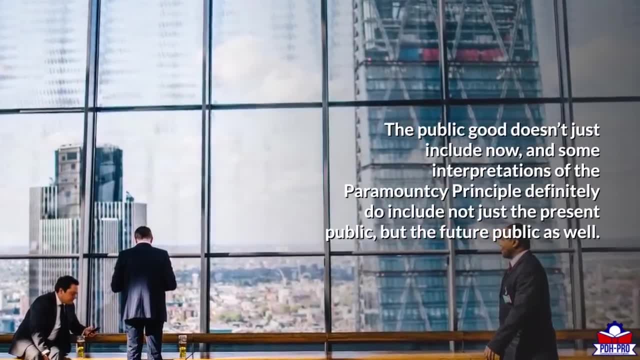 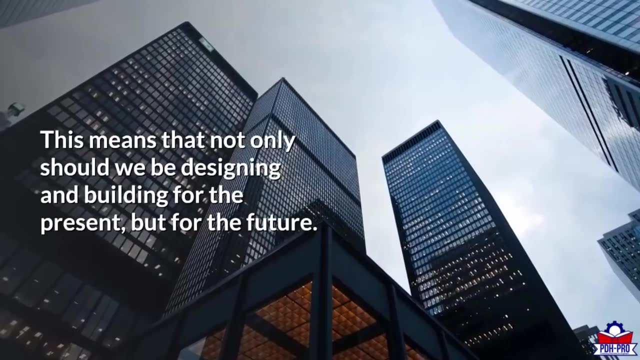 many think about the public. good doesn't just include now, and some interpretations of the paramount principle definitely do include not just the present public, but the future public as well. this means that not only should we be designing and building for the present, but for the future. this brings environmental concerns to light and makes us think about the 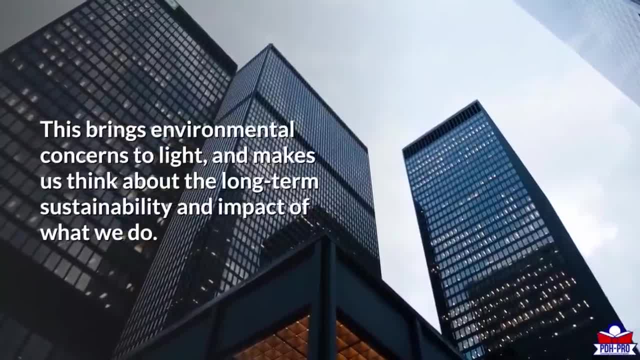 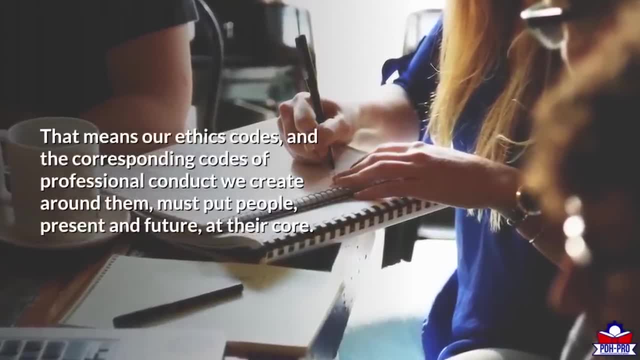 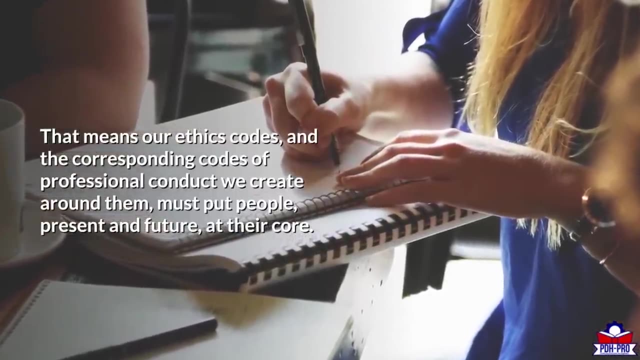 long-term sustainability and impact of what we do. the whole of the paramount c principle is the present with an eye towards the future. that means our ethics codes and the corresponding codes of professional conduct we create around them must put people present and future at their core. we'll find ourselves not only with professional jobs but also with the